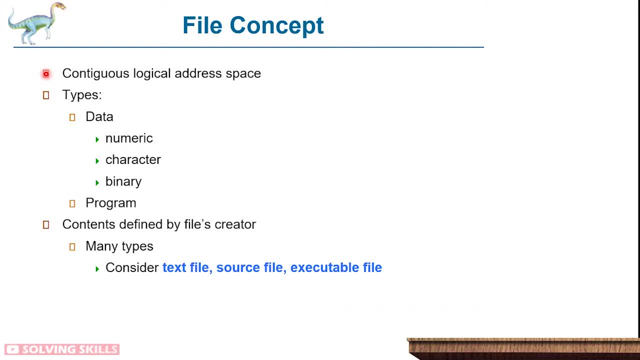 earlier that there are logical units, logical blocks inside the storage media and these are contiguous, meaning they start from zero and then one and two and simply they go on and we don't worry about where they're stored physically. and the files? uh, the file can contain data or it can. 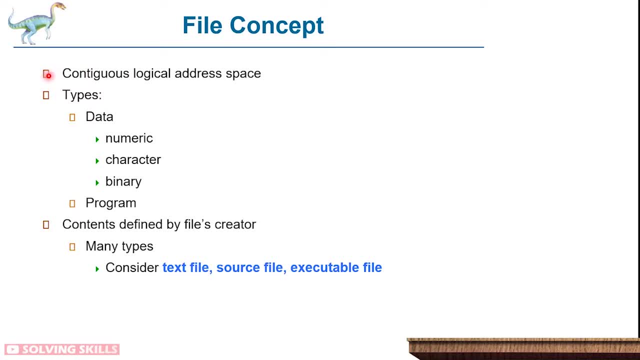 contain a program. the file is a collection of contiguous logical address space, right so the blocks number, block numbers that we are talking about. so if you collect a group of block numbers, that group can be called the file. so, and the contents of those that file could be either data of numeric type or character type or simply binary type. binary type. 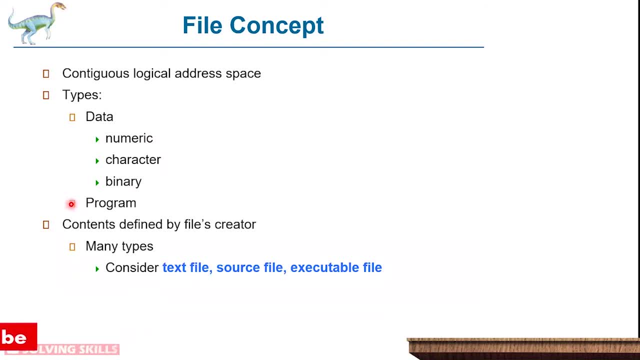 or it could be a program that could have instructions that can be sent to the cpu, or first it will be loaded to the memory and then sent to the cpu. the contents defined by the files creator could be of many types, like text file, source file, executable file, because in the binary 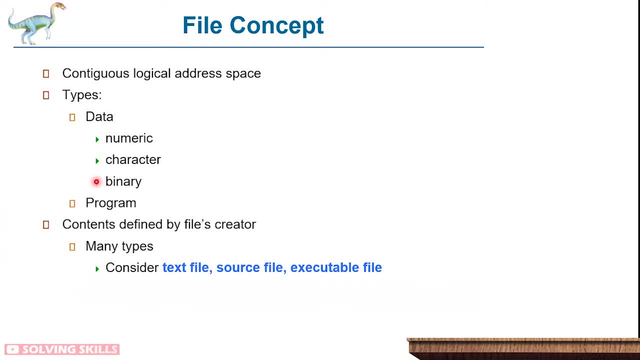 format. you are able to define your own file format to have your program read data in a specific format that only your program understands, right? so, so that allows for, uh, infinite number of file types that you uh can create, and uh, so there are some attributes that each file has. the first 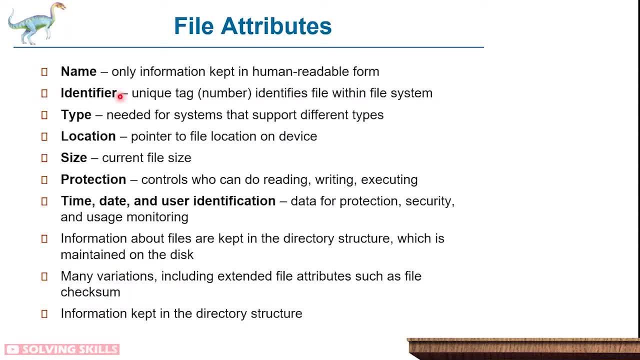 one is name, and then the identifier, which is the unique tag which identifies the file within file system. right, so, uh, these are two different things, because, uh, the the file is a physical entity which physically exists on uh the surface of this physical media somewhere, but uh, the there. 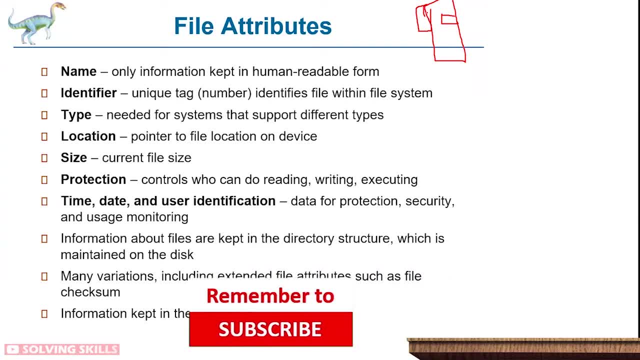 is a separate thing stored on on this physical media, which is the managerial information about, you know, uh, all of this data data, about data that will have to know the identifier for this file in order to- uh, you know, access the file instead of the name. so it is just like a program name was a file name when we studied programs and the pid is its. 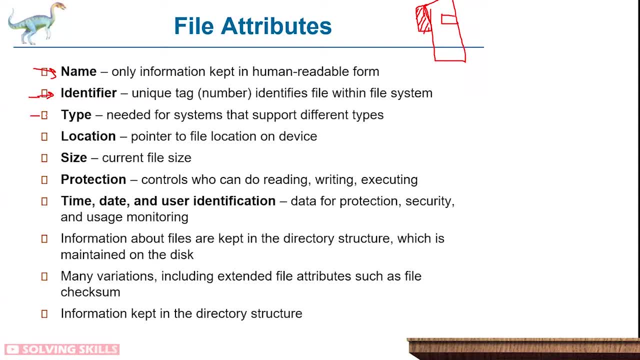 identifier number. just like that, we have a file identifier as well. then there is file type, then file location, then file size and then the protection information, like who can read, or like user rights to the file, and then there are time and date and user identification. all of these 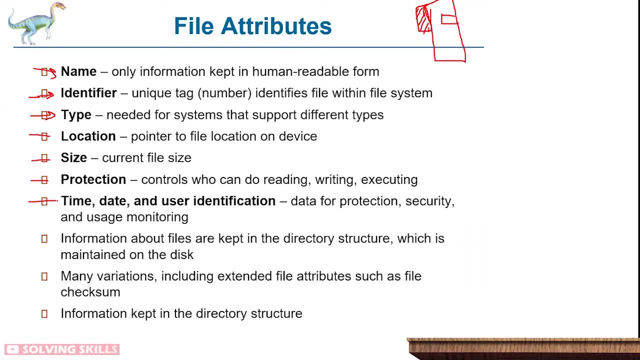 kinds of stamps on the file which tells you, uh, when the file was created, and then you can see the data that was created and when it was modified, etc. and information about files. uh, yeah, so these things are slightly different. so all of this information about the files, where it is stored, 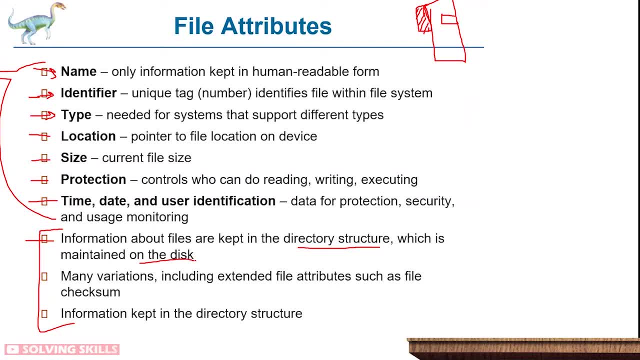 it is stored in the directory structure which is maintained still on the disk alongside the files. many variations, including extended file attributes such as file checksum. so these kinds of attributes allow you to check the files for uh errors and the security of the files. so this is all part of the directory structure. so this is the main. 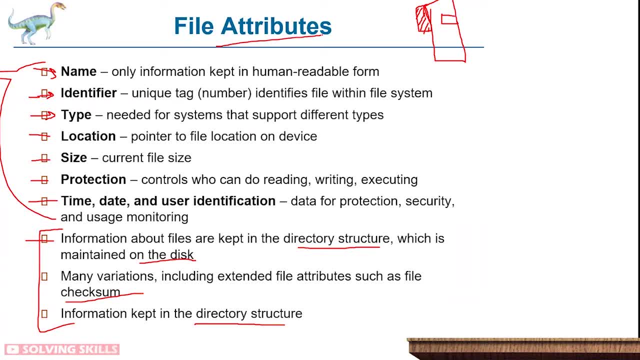 location where all the information about the files uh is stored: which, how many, which logical number, block numbers uh this file contains and what is the name of the file, what is the id of the file, what is the type, location, size and other information of that file. these are all stored in. 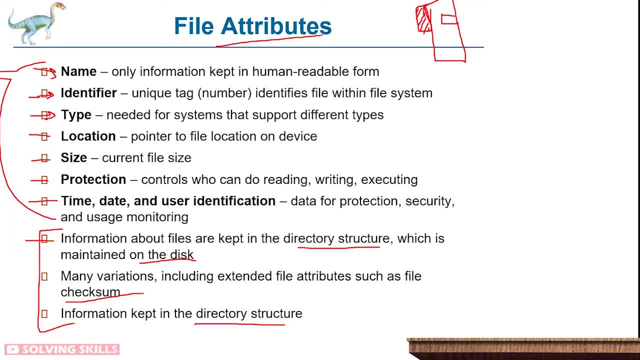 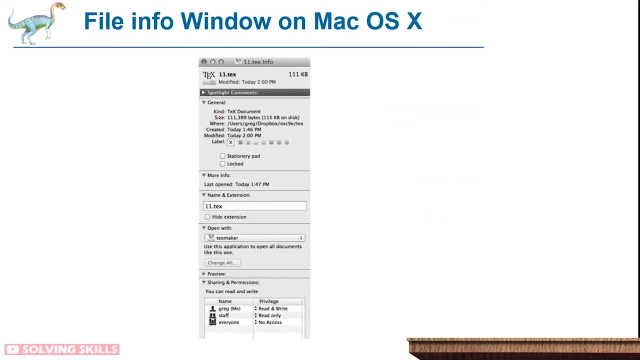 the directory structure how files are grouped together inside a directory. this is also stored in the directory structure. so, as you can see that these are the attributes, like what is the type of the file and what is the- they call it kind over there, and then what is the size, where it is stored inside the directory structure. 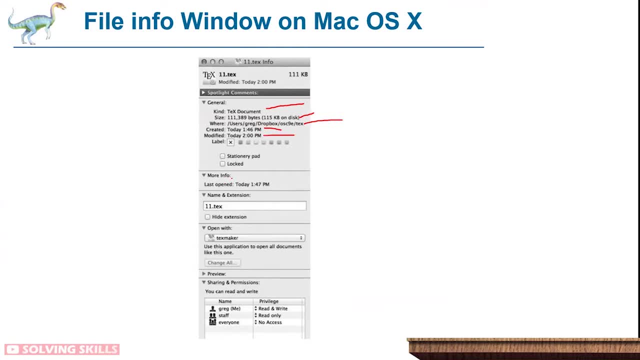 when it was created, when it was modified and similarly, there will be some privilege information like the access permissions, like who is able to read and write to the file, who is able to only read to the file from the file, or who is who can access the file. so, similarly in windows, 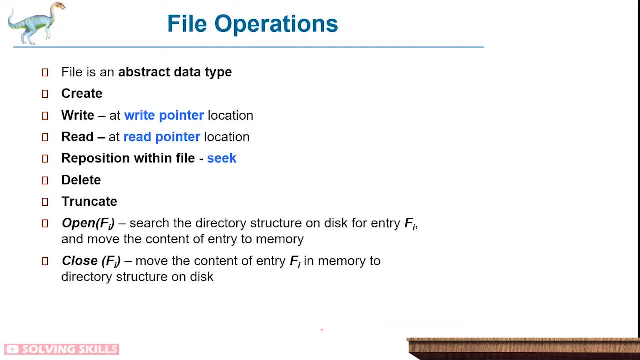 there is a similar, you know, attribute windows and, similarly, file operations, the operations that we perform on files. we can create a file, write, read, reposition within file, delete, truncate or open or close the file. so these are different operations. very obvious, because file is an abstract data type, because it contains of logical numbers and that's it. so when you ask the operating system, 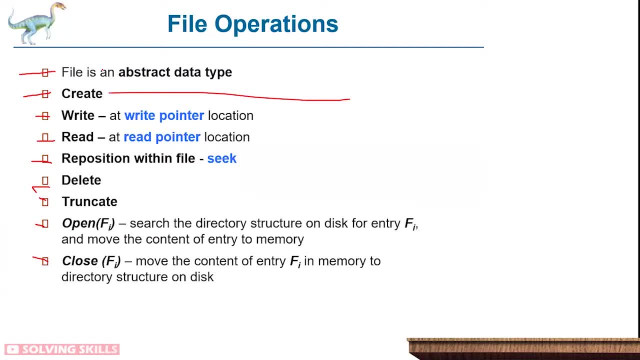 to create a file. it is going to find p logical blocks on the surface of the storage media and it is going to create a new entry inside the directory structure that i'm going to allocate these logical blocks to, to this newly created file. similarly, you are able to write to this file or: 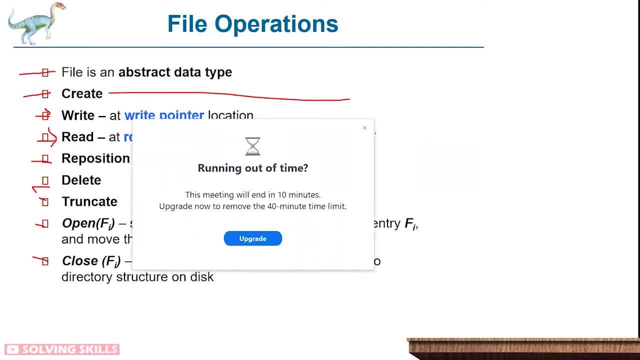 read from this file and by the way these read and write operations, you have to use the intermediate interface of memory for that. so all the data that you request to write first goes into the memory and then the operating system is is responsible for taking that data from memory into the disk to the desired location. 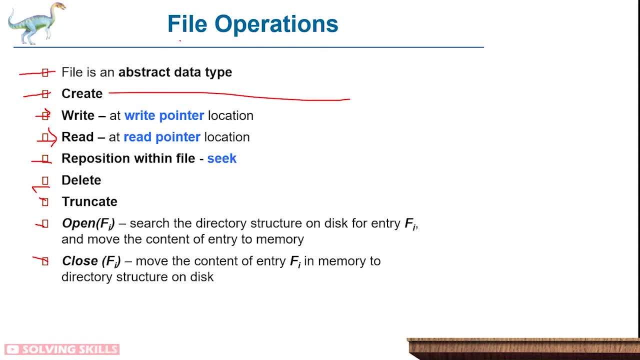 where the directory structure is pointing for the logical blocks of that particular file. similarly, read operation is similar and all the data from the disk is going to be read by the operating system to the memory based on any read or write pointers which point to the logical blocks of that file. 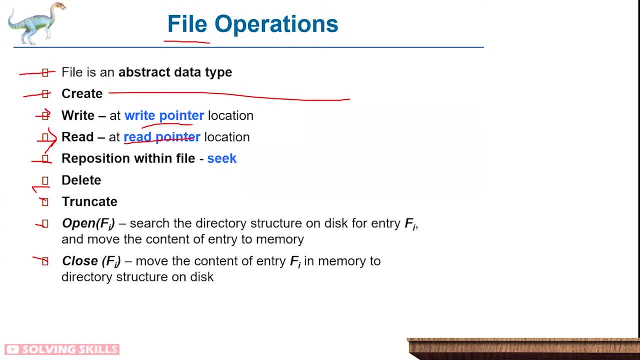 which are already, as i said, are stored inside the directory structure. so, similarly, you can reposition within, within the file, just like, for example, in the cassette players from the old days. you know that you, you had to, you know rewind or forward the amount of you know tape. it is like 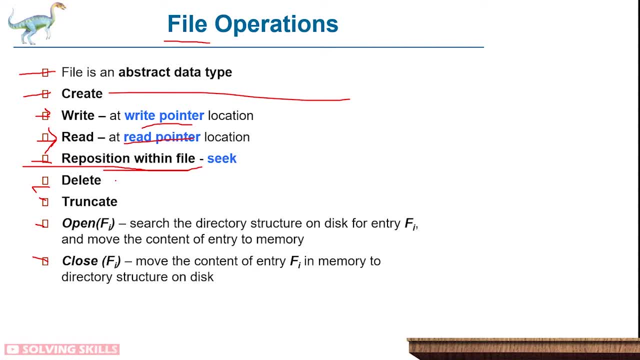 repositioning your head on top of that magnetic tape and similarly you are able to delete the file or, you know, change its end, location, truncation, and similarly you can open the file which brings the file into the memory, or you can close the file so that it is backed up on the hard disk again. 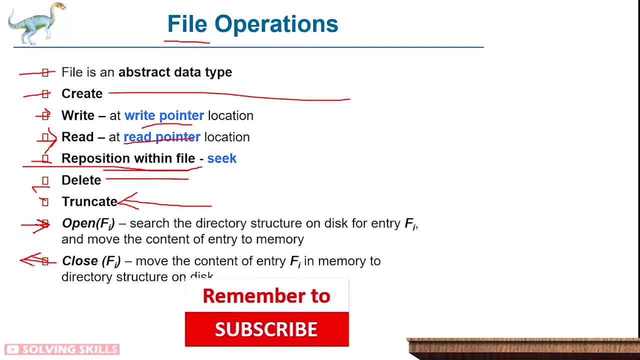 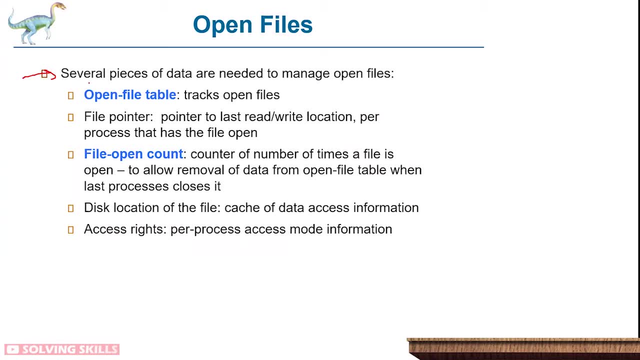 and it is closed from memory or remove, removed from the memory. so whenever multiple files are opened inside an operating system by different processes, the operating system maintains a open file table to track the open file. so for example, in the operating system right now there are 100 files open. so the operating system is going to maintain an open file table and there 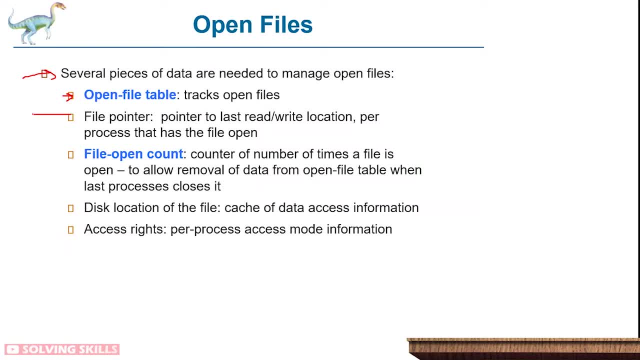 will be a file pointer which points to the last read write location per process that has the file open. it is just like the program counter that we saw in the processes part, so just to keep track of where you've the last time a process accessed this file, the file pointer is directly in the process. and during theанию process, when you don't have the file put in, receive it- and here if you make the files go away, go with, the process can be trapped- should be stopped. so something like this, or if normal, blame on yourself or something like that, that's what called thelave test Your machine would ask for. 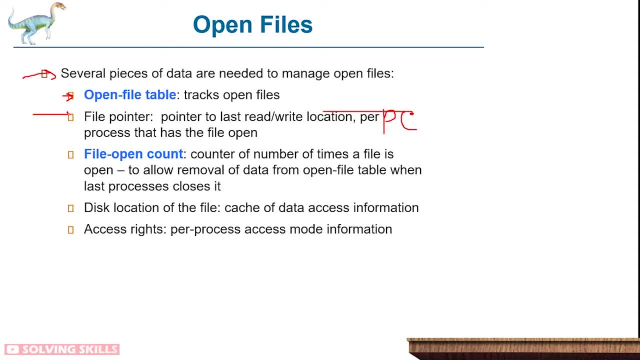 because the state of the process that is now comfortable for self- 않고, this property of object data need to be行 of responsibility. that's what what you mean for account of the. the process here is to safe on the file, and they home will point to that. and similarly, file open count is the number of times a file is opened by. 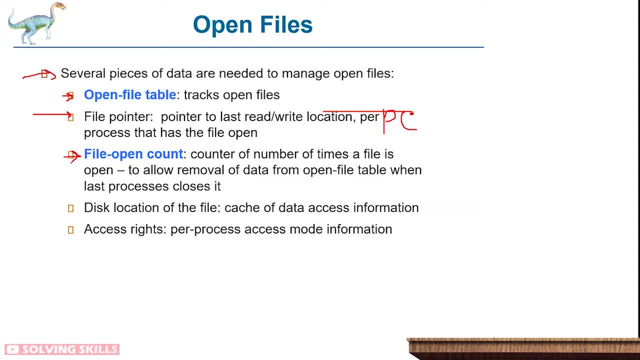 different processes, so, for example, multiple processes. there's a read-only file and multiple processes are reading this file and similarly this location of the file cache of data, access information. so the directory structure is going to be cached into the memory for faster access to the disk and similarly, access rights will also be maintained about the open files, so that it's 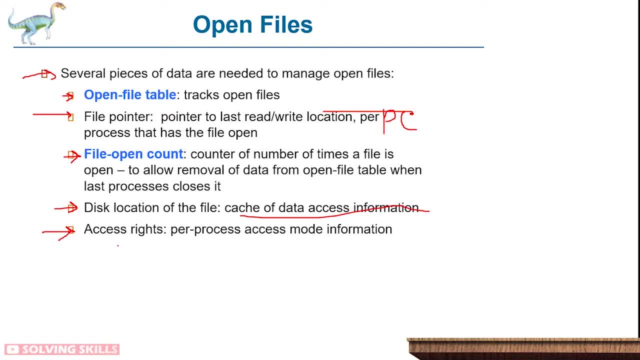 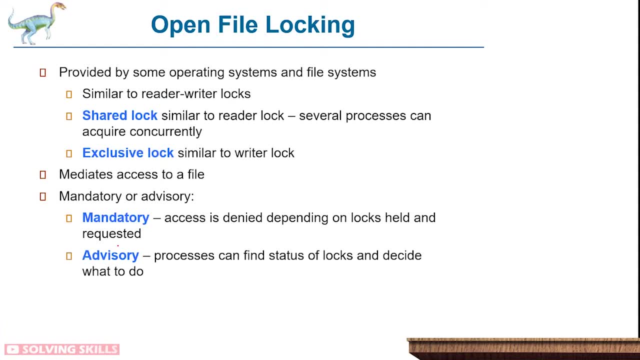 easier to protect the files from invalid access. so this is all we do with the open files. and then, of course, there, because open file- an open file is- can be a shared data, so you need to apply locking to that so you always see that, for example, you are accessing a file inside the 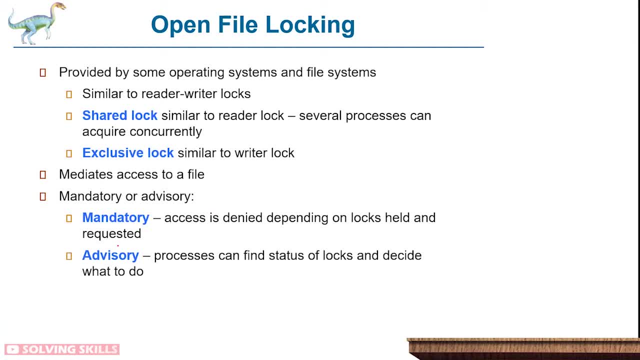 microsoft word and you are trying to open the file in some other. uh, you know, you know doc in other applications. so the application would say that this file is already open in some other opera. you know process, so i'm not able to open this file. so that is the locking mechanism. 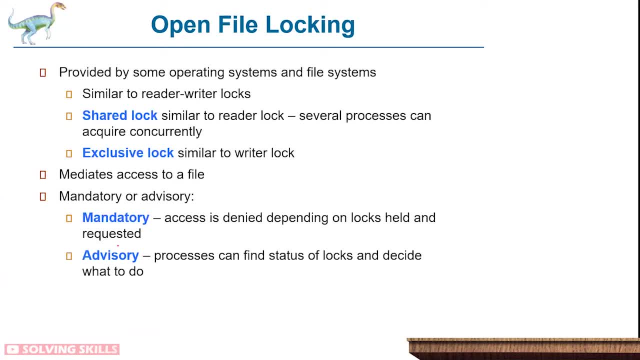 just like we saw in the synchronization chapter that you can have, you know, semaphores or mutexes that allow access to a shared data. so those locks are also implemented for the you know. so here they say the share data. so those locks are also implemented for the you know, uh. so here they say the share. 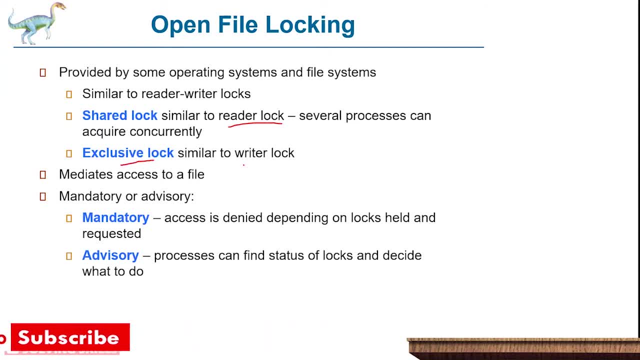 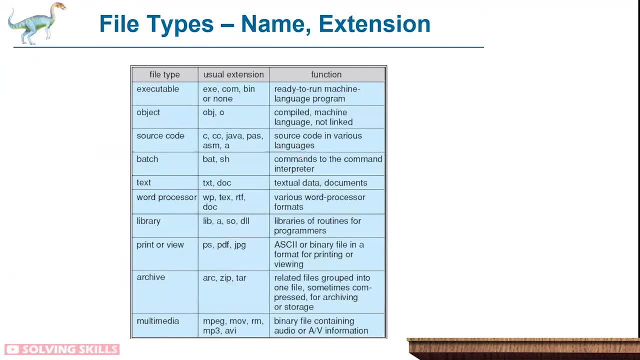 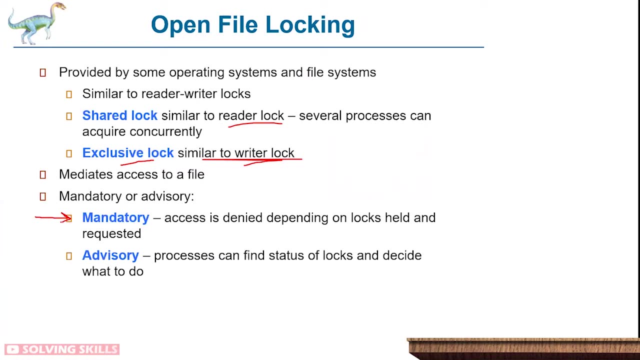 shared lock is similar to reader lock and the exclusive lock is similar to writer lock. that we already studied in the synchronization chapter. so sometimes it is mandatory. for example, the file is when you try to open it multiple times it will deny access, and sometimes the lock is advisory that you are allowed the opening the file in multiple locations multiple. 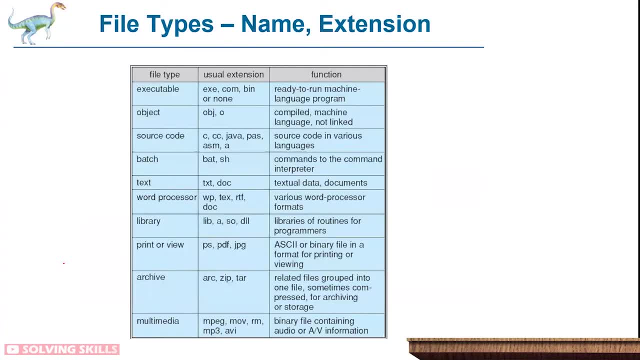 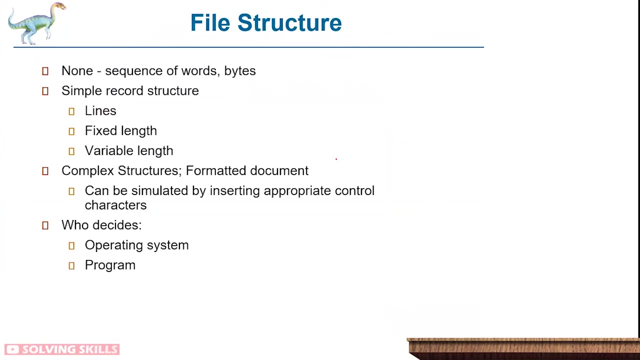 processes, but it warns you that you know it is not advisable to do that. then there are so many different types that you always see inside your operating systems, like the txt file or maybe jpg file or avi file, or so we see all of these files so many times when you're using- we are using the. 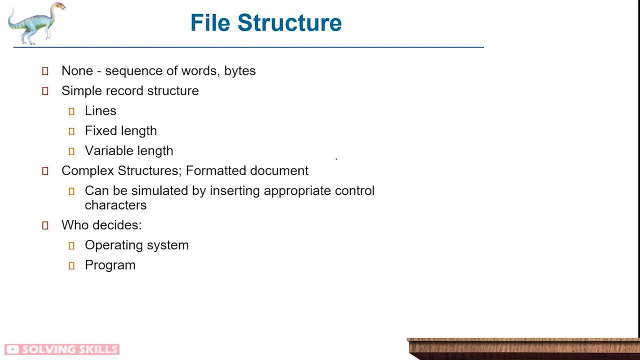 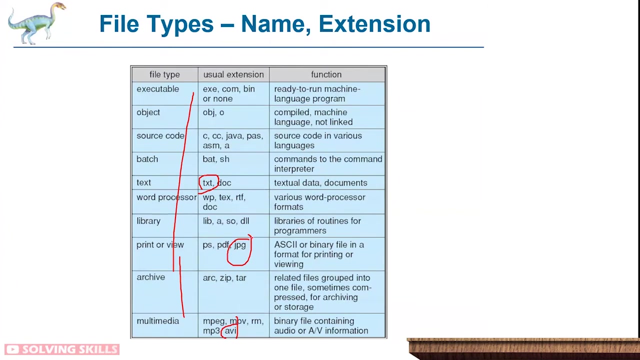 operating systems. so then there is file structure. so if there is no file structure, then it is just a sequence of words or bytes and you are responsible for deciding which part will represent what. so, for example, when you study the, you know, I just recall that- when you study the format of jpg file or avi file or txt file. so the first few bytes, 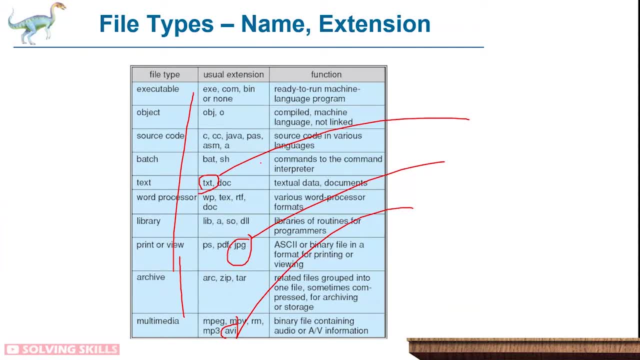 inside these files. they represent different kinds of information about the file. for example, in the jpeg it tells you the compression information and different types of uh. you know information that what colors are being used in the image. it is also stored at the beginning of the file. and uh. you know what is the resolution of the image. 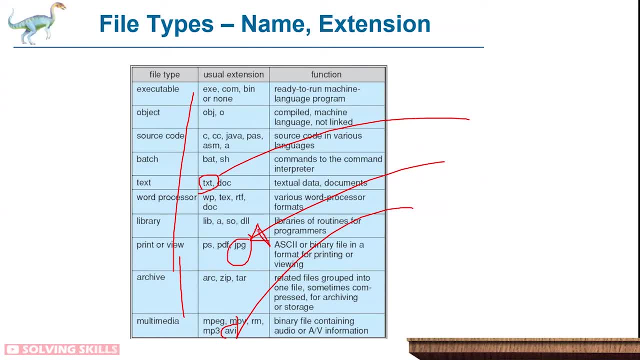 what is the size of the image. so all of these informations are stored at the starting of this jpeg file. so uh, also called the header information. so the header information is only part of the data file, but the but because we knew that it's a jpeg file, we know that there. 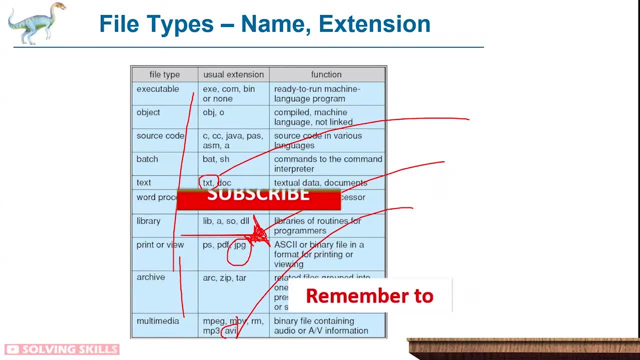 is a standard way of storing jpeg file and the starting location. the starting bytes are going to tell information about the data, so also sometimes called metadata. right, so it's data about data. so, but, but, but from the perspective of a, you know, physical storage. there is, it is not different, any different from you know, simple bytes. so these are. 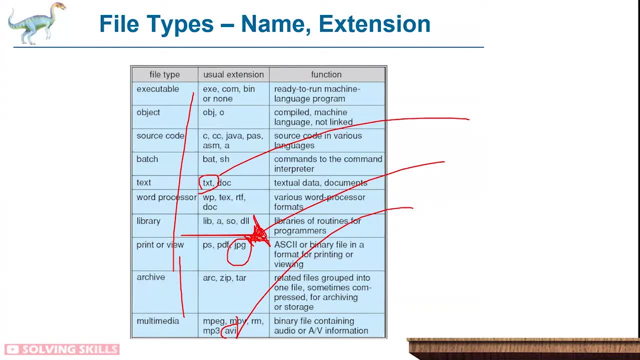 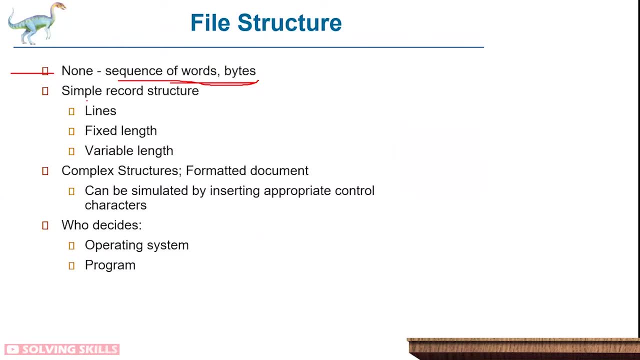 simple bytes, but they represent something that we know. we have a priori knowledge of what those bytes represent, right? so simple? uh, then they are simple record structures, like lines, fixed length or variable length, and then their complex structure, which are formatted documents like, as I told you. 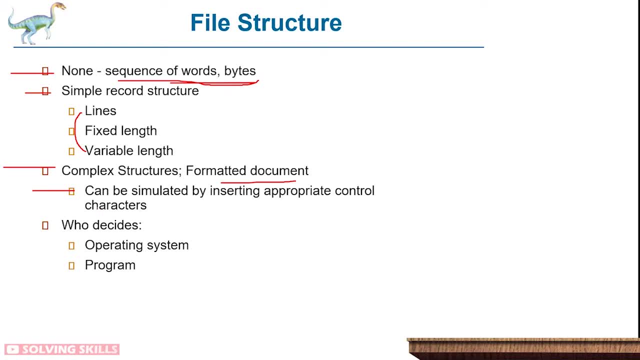 jpeg can be simulated by inserting appropriate control characters uh the structure, the operating system and the program. so the operating system uh would definitely decide the file structures for the file types which are well known, which are used by the users and the operating systems alike. so the operating system is going to uh give some kind of documentation. 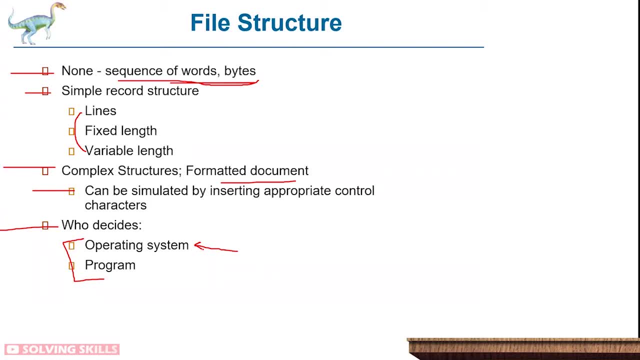 or tell you that this file type should have this kind of structure inside, but most of the times decide which. what would be the structure of the file, right? so we see new file types emerging every day. actually, it's really easy to- for you as well- to write a program which you know defines a self-defined 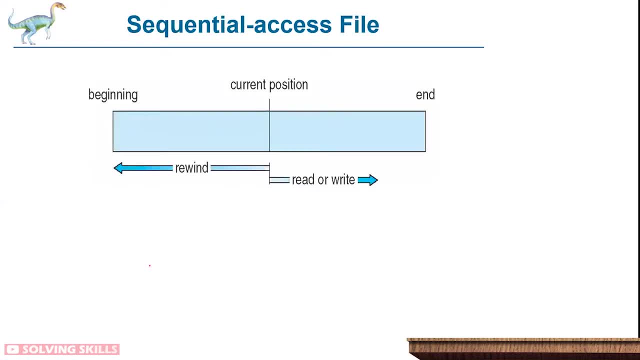 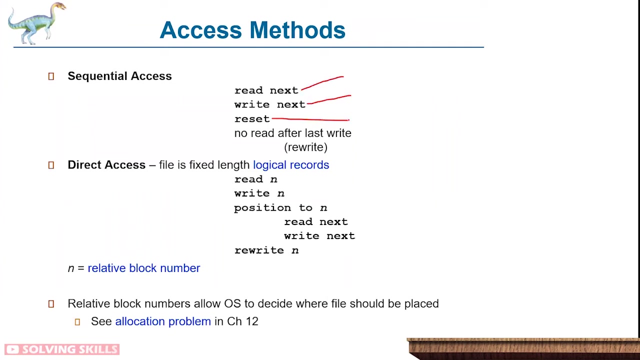 type and then manipulates the data accordingly. so sequential access file is something when where the pointer points to one location and you simply, uh, tell the pointer to go forward in one direction or reverse into another direction. so for that the system calls are simply like read next or write next, and then resetting takes you to the first. 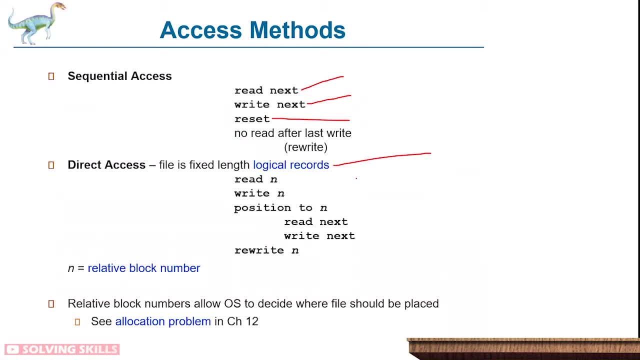 starting location of the file. and then there is direct access, uh, random access you can also call it. it simply tells the operating system to read the number, the actual number of the block that you write to which block or position your head to which block, and block number, and then use the sequential. 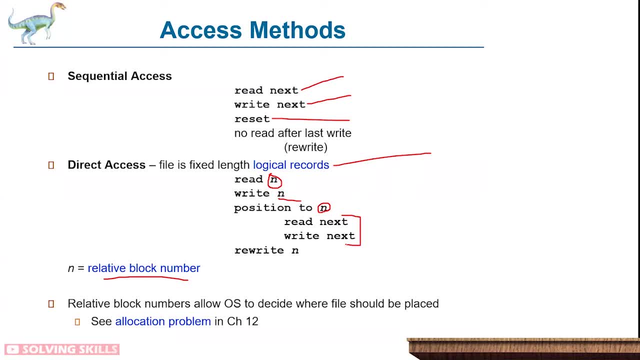 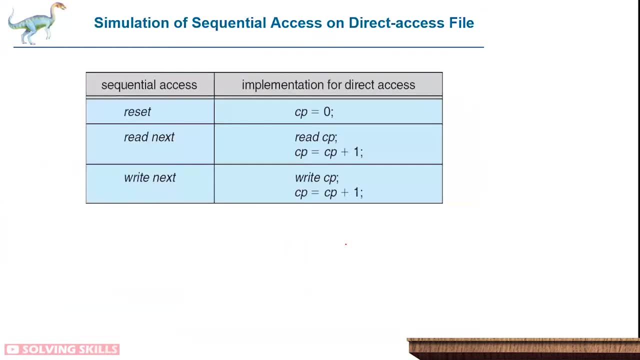 access type which is read next or write next. these are really, you can say, logical or obvious kind of mechanisms to read or write to files, and so this is how you read next: you simply read the current pointer and then you increment the current pointer by one and if you write: uh want to write to next. 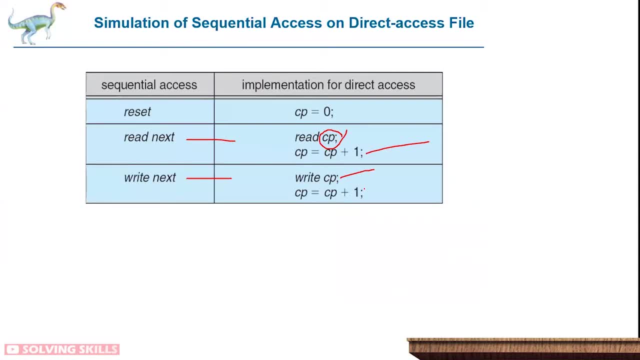 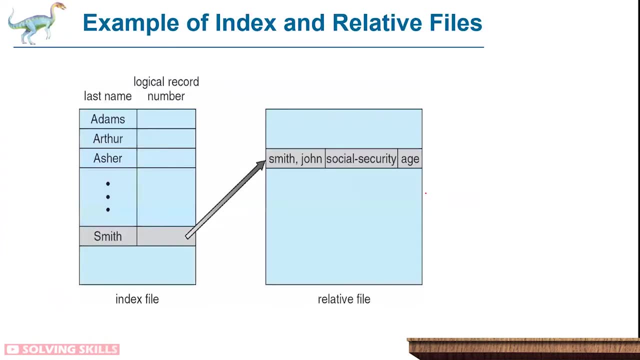 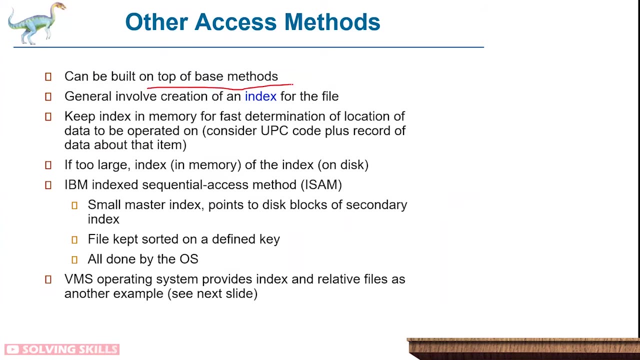 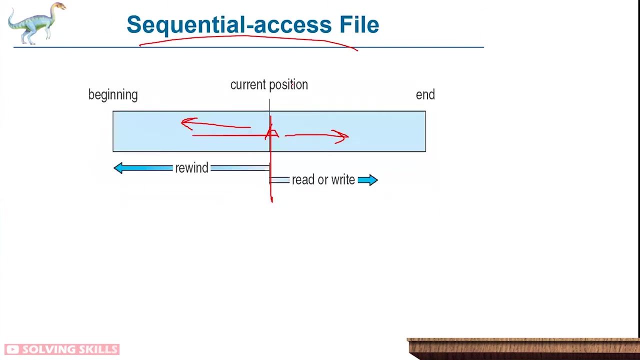 block number. you simply write to current pointer and then you increment the current pointer to go forward. so other methods, other access methods, are one of those are called, and they are built on top of base methods like this, this: these methods may be the lowest level methods that are implemented to 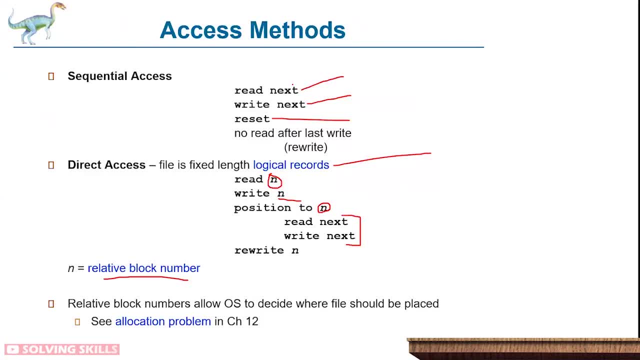 access logical blocks. but on top of those, using those uh- you know- base level access methods, you can define higher level of abstraction to access uh logical blocks, so you can visualize your blocks as a tree or as an array or as a two-dimensional array. all of those methods can be implemented. 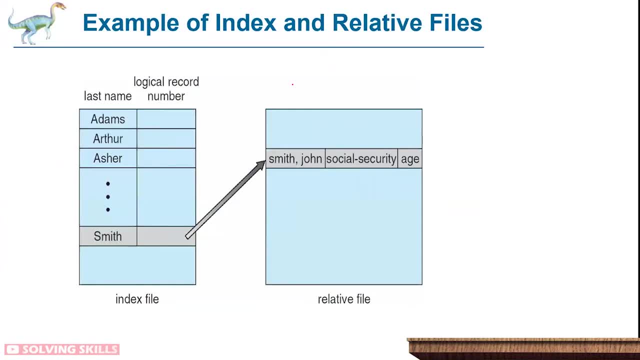 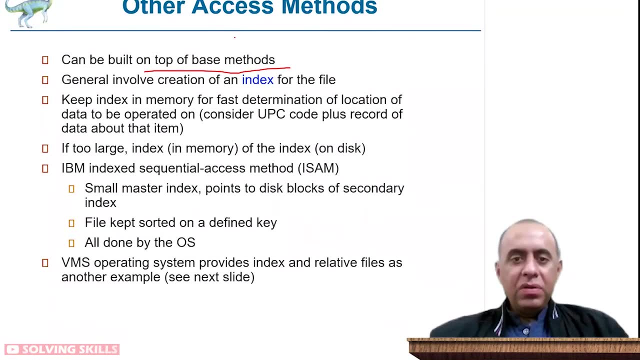 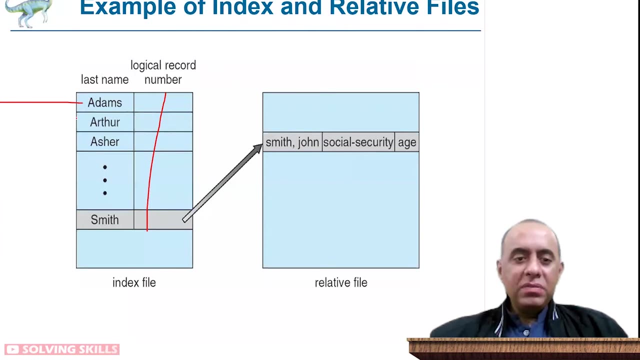 using these base methods. so let's look at those. the first one is index. for example, you wanted to create a file that, uh, you know, contained these kind of records like uh would be last names, the. so all the records will be sorted with last names and there will be logical record number and for each record number there would 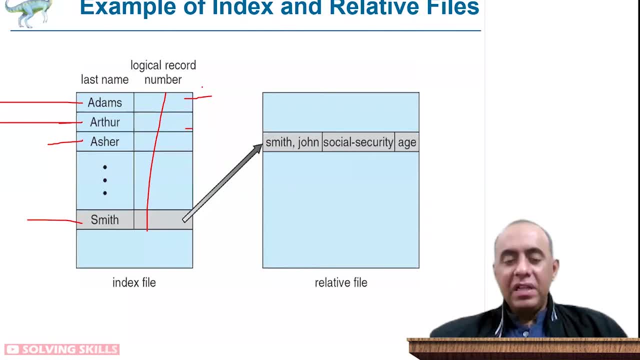 be separate files. so the file that saves the records is called the index file, so it provides indices to the relative files and when you go from one index file to the relative file, inside the relative file there is going to be more information about that record that you wanted to access. so this, this would be: 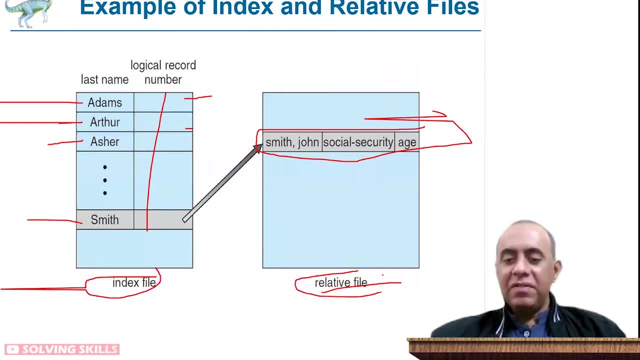 so these are two separate files. the index file and the relative file are two separate files. this is a, you can say, a higher level access method for to read files and similarly the directory structures. so so this is only one example of a higher level of abstraction for access methods: the directory. 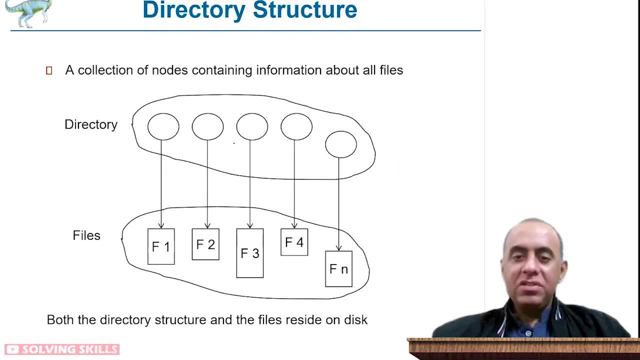 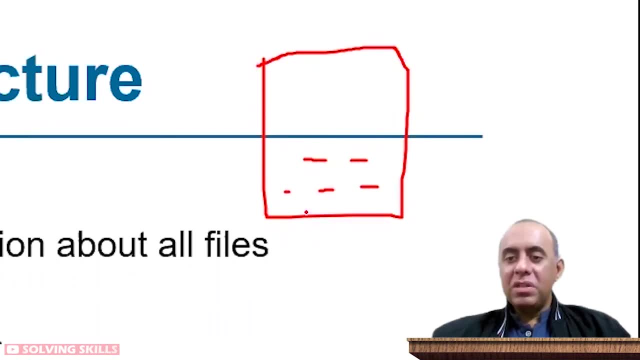 structure itself. it is slightly different thing, which is again, as I said, this is your disk and inside the disk there are different logical block, block numbers. how does the operating system know, and who will tell the operating system which logical block numbers? for example, I say that these logical block numbers are one file right. 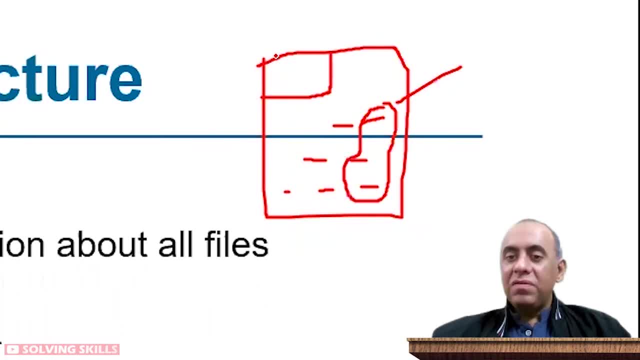 so there will be a kind of record management system on the disk as well, on a disk in a in the corner of the disk. and the evidence for that is that whenever you buy a storage device and you try to write to that storage device, so when you 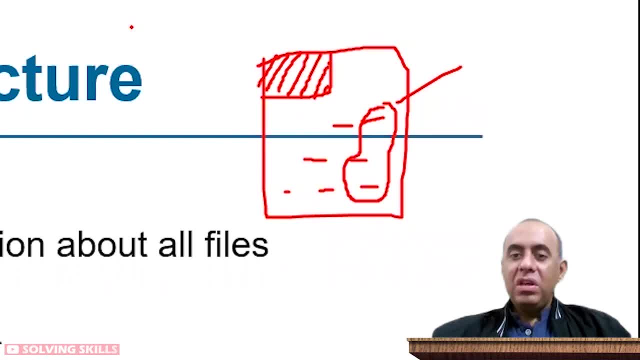 try to access the files. you can only use slightly less amount. then you bought the disk for for a terabyte disk. if I bought a disk of 1000 gigabytes, so I will maybe get 970 gigabytes of data. so where did you get the data data? the data was just. 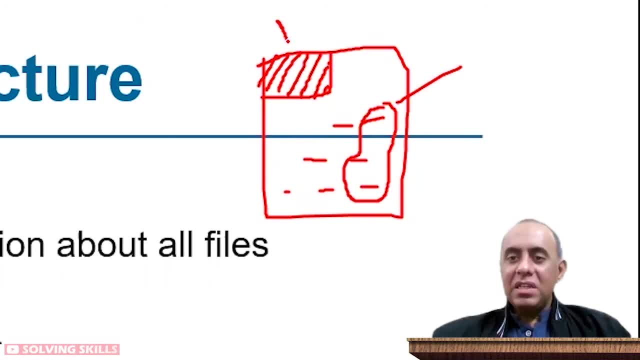 the 30 gigabytes of data go. that 30 gigabytes data actually went to the directory structure, right? so because it is in storing the information about 970 gigabytes of these blocks, so that will be called the directory structure. this thing will be called the. 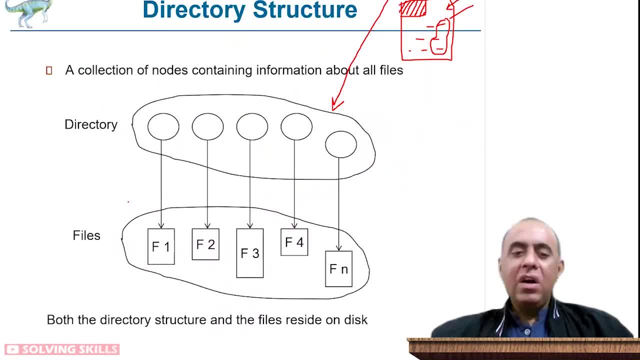 directory structure. so the directory structure will contain all the information about files. for example, this file contained like 100 logical blocks, so all those logical blocks, starting from the first one, will be stored inside the this logical, this directory structure and in one way it will be pointing to that file, right, so you can say: this is this directory structure is. 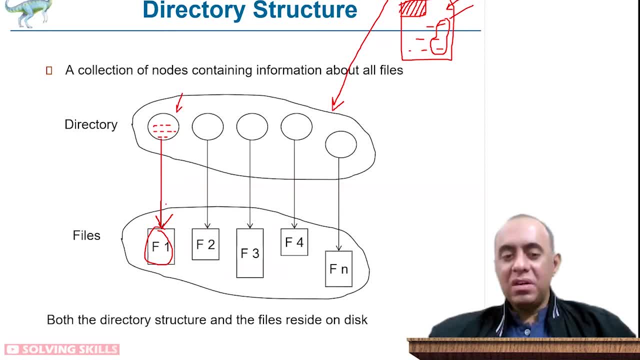 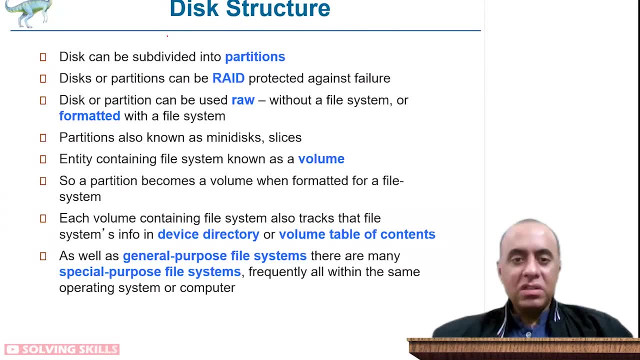 this node in the directory structure is pointing to this physical file on the disk. so in order to you know, elaborate the directory structure, first we need to know what disk structures are. this disk can contain multiple partitions and they can either be used raw or they can be. 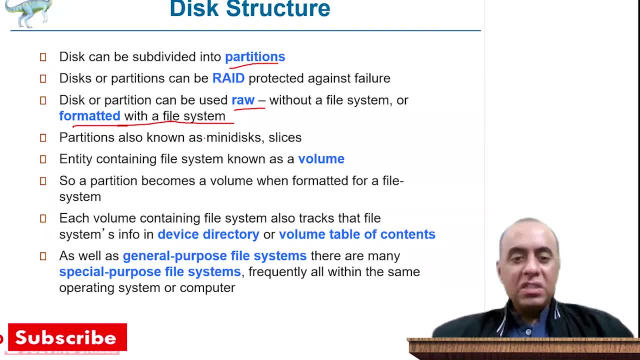 formatted with a file system. so partitions are also called, or they can be known as mini disks or slices, and every entity containing file system is known as a volume. so there's a. the difference between a partition and a volume is that a partition may not contain a file system. it may. 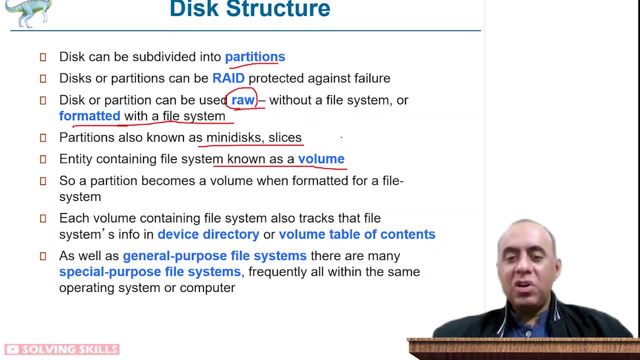 be raw, but when you write a file system on it it becomes a volume. so these are just traditional names for these things. so per partition becomes a volume when formatted for a file system. so each volume containing file system also tracks that file systems. information in device directory. 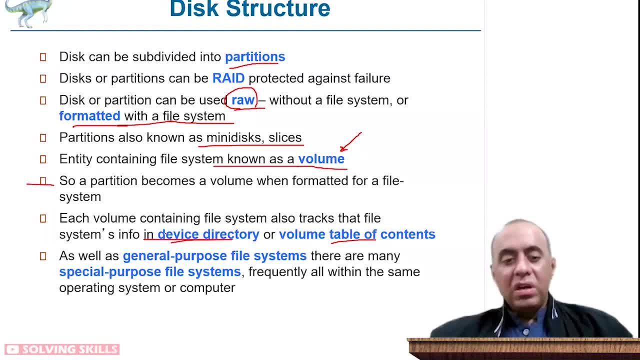 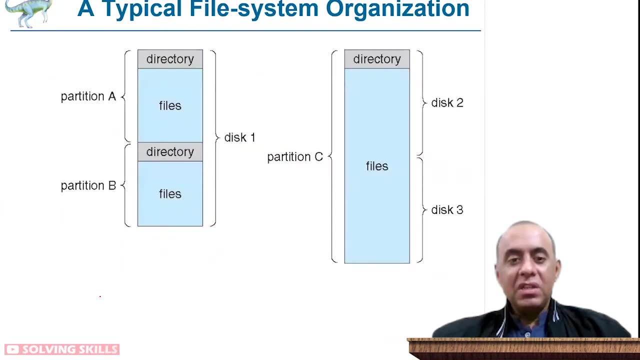 or volume table of contents. so these are again, as i said, names for you know, supporting things to the directory structure and as well as, as well as general purpose file systems, there are many special purpose file systems. so let's have a look, and this is the picture for one. 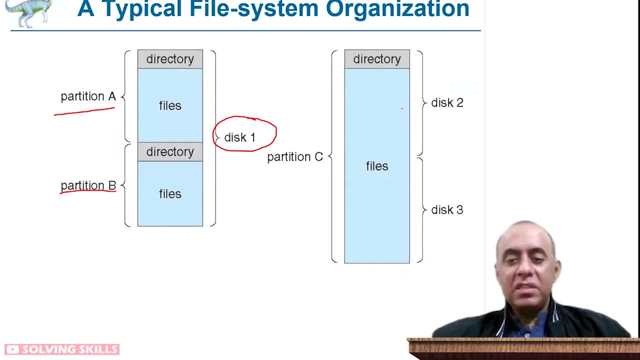 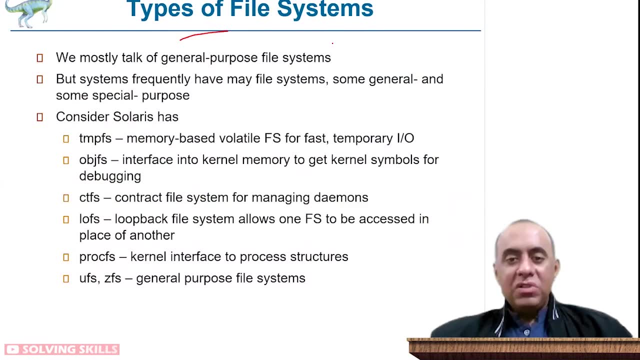 physical disk divided into two partitions, and this is the example of two physical disks combined into one partition. so these, both of these things are possible. and then the types of file systems. uh, these are different file systems and, again, as i said, uh, they are different. like, for example, there is tmpfs in solaris. these are all solaris file. 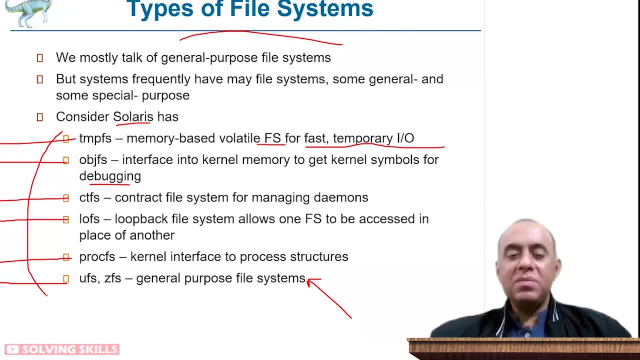 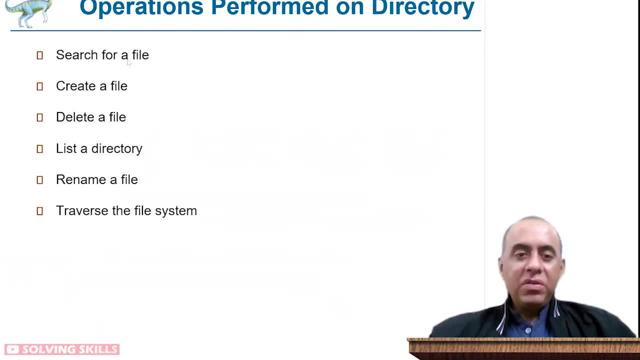 systems. these are all special purpose, you can say file systems which are defined by a particular operating system, so operating operations performed on the directory. you can search a file for a file inside the directory structure. you can create a file, uh, so, as i said, so if you're searching, 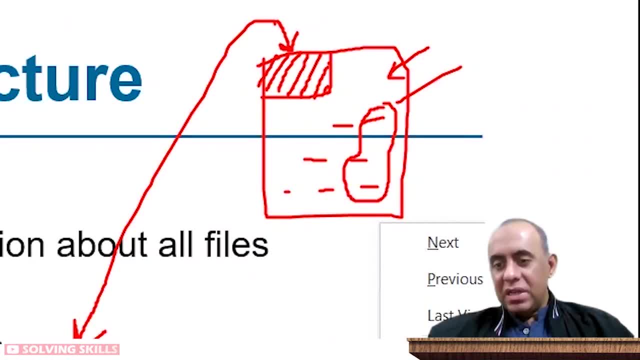 for a file inside the disk. if i ask you guys, what do you think? will we be going into this for this part, or will we be going into this part? so, for example, this was a one terabyte hard disk and 970 gigabytes were over here and 30 gigabytes were over here. then the searching is done in the 30. 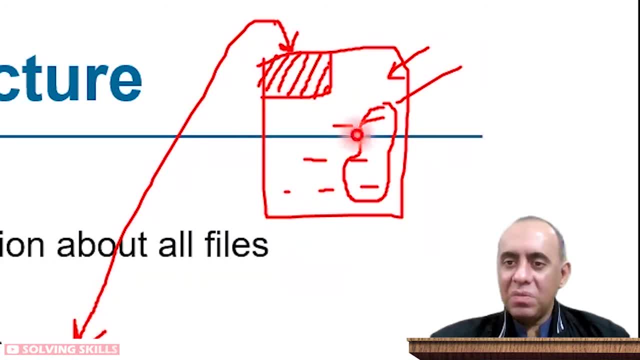 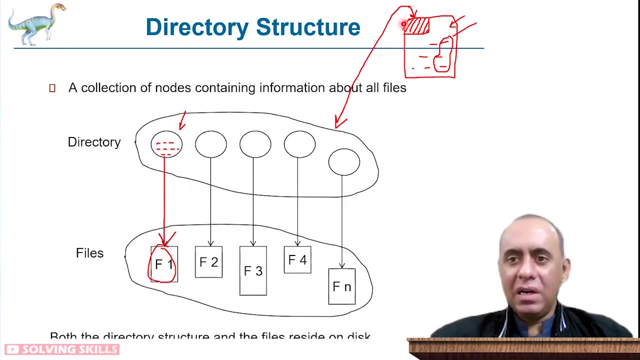 gigabyte area, which is the, the information about the files, and you just need to look in for names or file sizes so you may have done file search. so all of this will be done inside the inside this, uh, the, the directory structure, so you don't need to go inside the data because, anyways, in going inside the data will be. 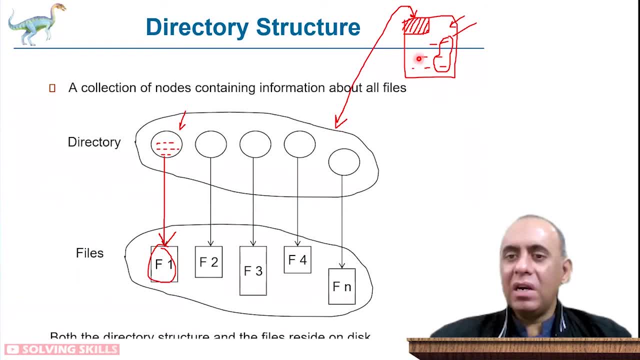 useless, because all of these, these logical block numbers, are absolutely looking the same, looking like they're just the same things, key repeated over and over again. the data inside will not tell you anything, anything at all. so, by the way, and that actually reminds you of the very important. 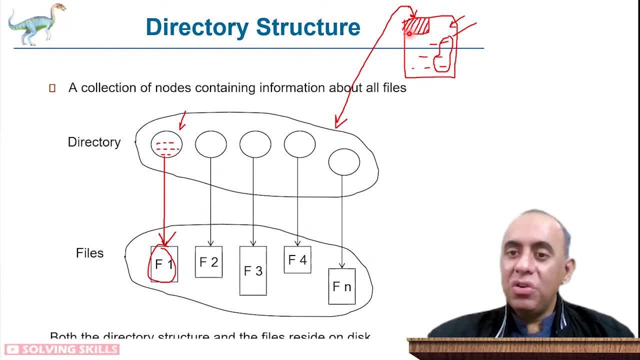 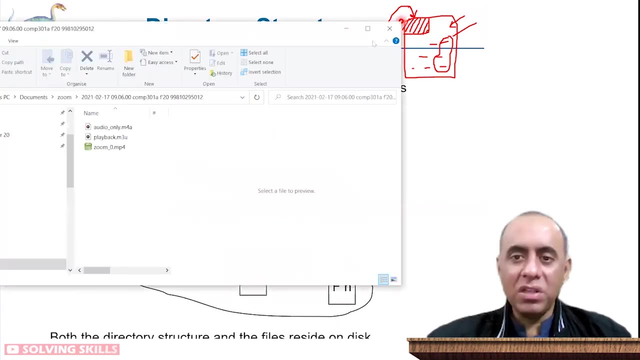 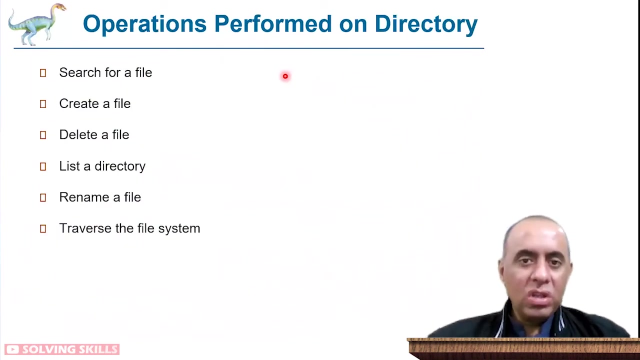 fact that if you somehow lose this data, your files, your files will absolutely become useless and they will disappear. you can never retrieve your files if you have lost your directory structure. so directory structure is an extremely important thing, uh, from that point of view. so, um, okay, so now the, the directories. you can perform operations you can. 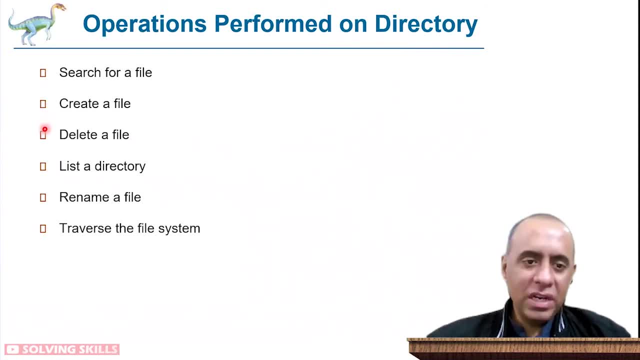 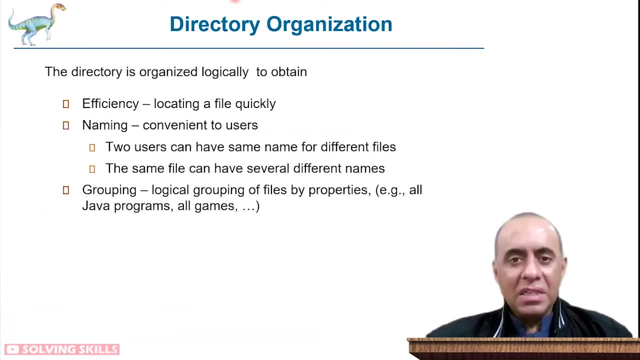 perform on directory. you can search for a file, you can create a file, you can delete a file, list a directory, rename a file, or you can traverse the file system and the directories are organized to for efficiency. like you, you're able to locate a file quickly yourself because you. 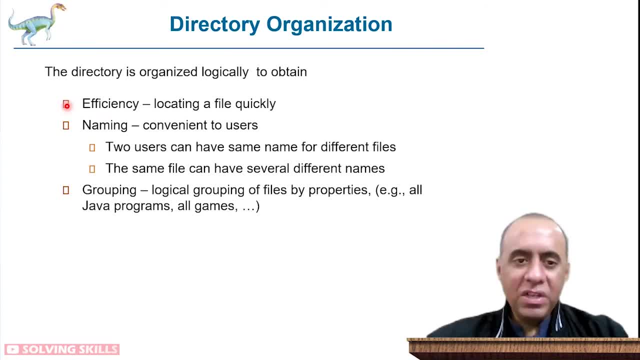 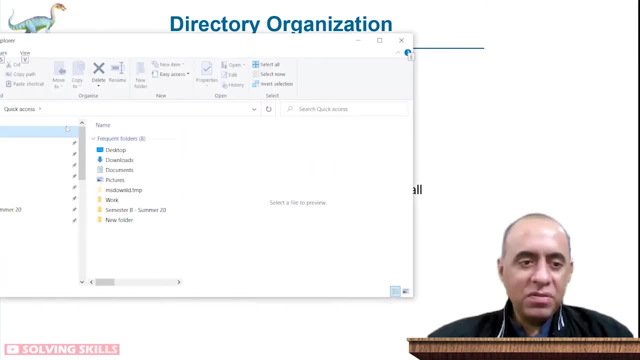 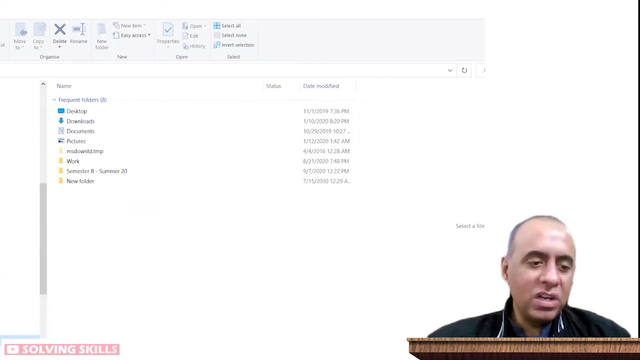 can see the, the directory structures, you can see which directories, uh, you can name them so that it's easier. like, for example, i have a work folder which i've been using for like decades now, because whenever i start this- any computer- so i simply go to this work folder and 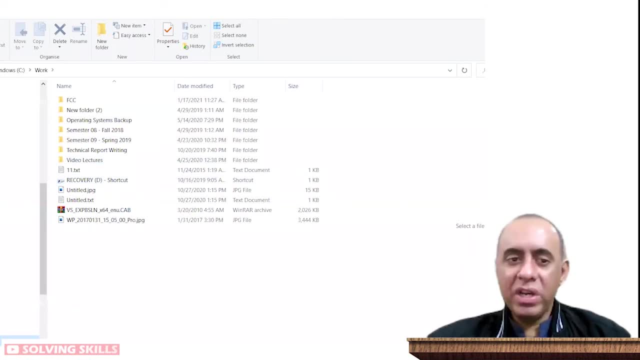 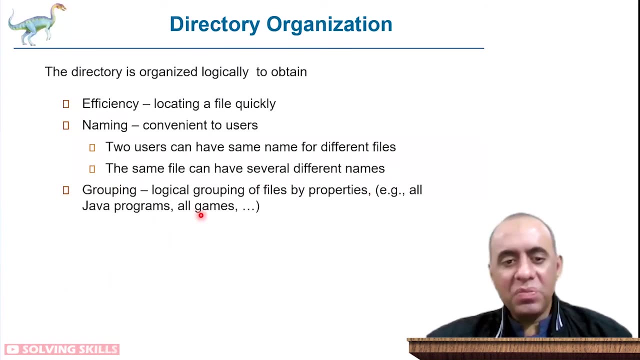 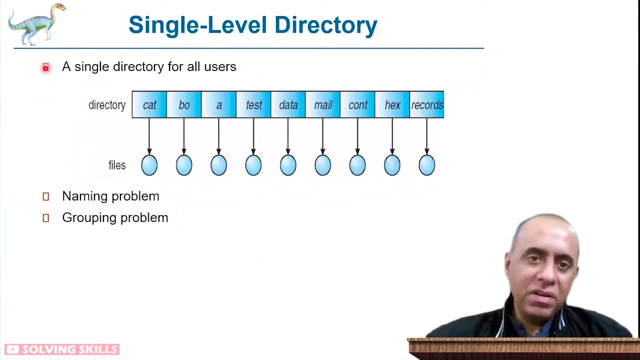 in the work folder i have like all of these different things that i've been doing and uh, then there there are grouping, like logical grouping, files by properties, for example, all java programs or all games. this is what you name just is also possible in directory organization and in the previous life of computers we used to have 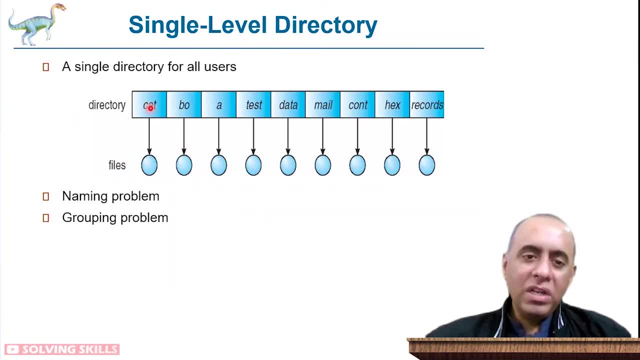 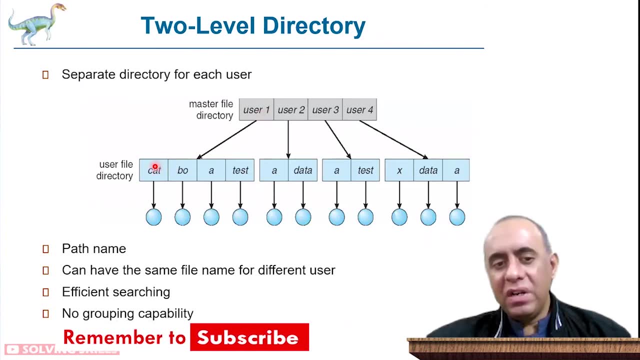 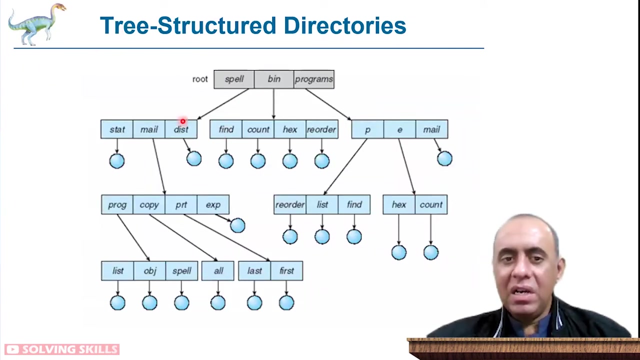 single level directory where one directory only contained one file. but but suddenly it became slightly different and we allocated different group of directories to different users and that work that was called a master file directory and the scheme was called two level directory. and then suddenly we came to the tree structure directory where we had sub directories and inside sub 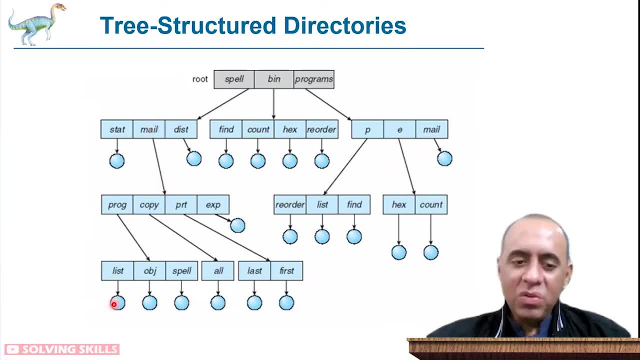 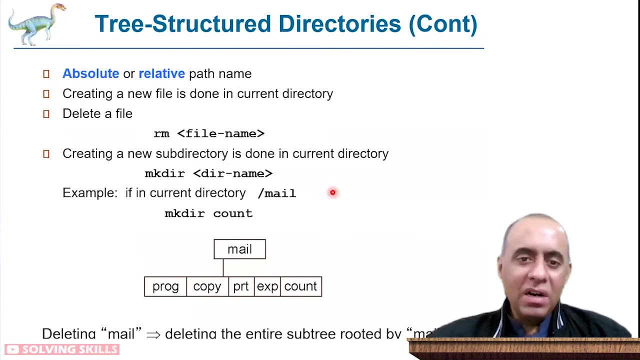 directories. we had multiple files and each file would be pointing to the logical blocks that it contains and sometimes, you know, even multiple directory locations could be pointing to the same. you can say physical files for optimization, and then you know these are different. you can say physical files for optimization, and then you know these are different. 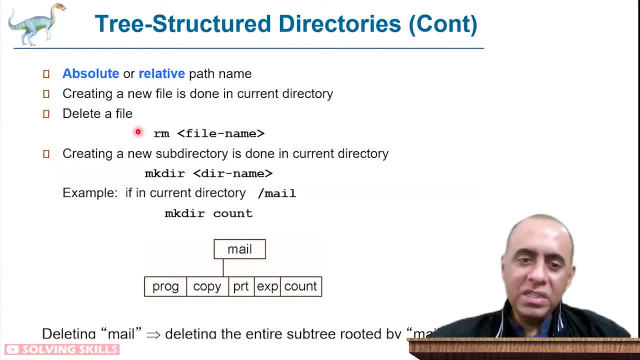 commands you use to modify the directories inside linux, like rm to delete a file, mkdir to create a directory, and you know stuff like that, and you already know the cd, which is change directory to navigate to different sub directories in order to access files. and then there are acyclic graph. 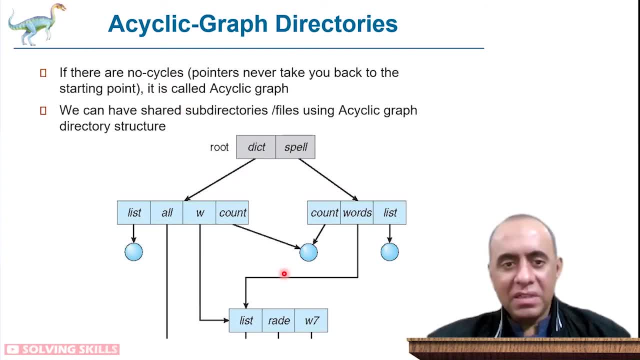 directories where you sometimes have cycles. so you you actually prevent cycles, but here you can see that the count type directory is pointing in both the, which are both owned by the dict directory and the spell directory. they're pointing to the same file, but this is not a cycle. this is. these are 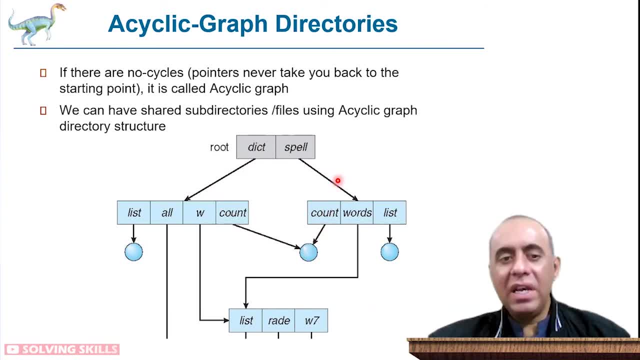 both ending at this node. so there is not like a reverse arrow here so that we can say that acyclic, this is the where there's no cycle, so we can have shared sub directories using acyclic graph directory structure. it allows for optimization. so, for example, this is a 500 megabyte file. 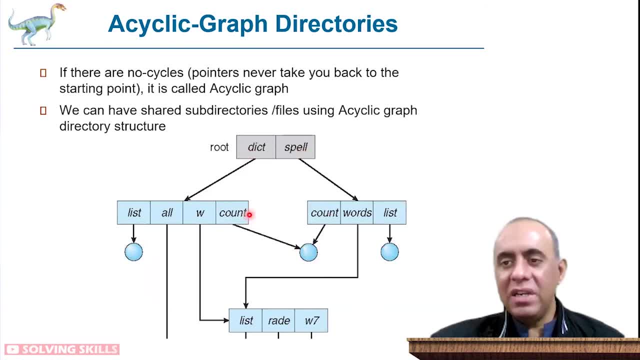 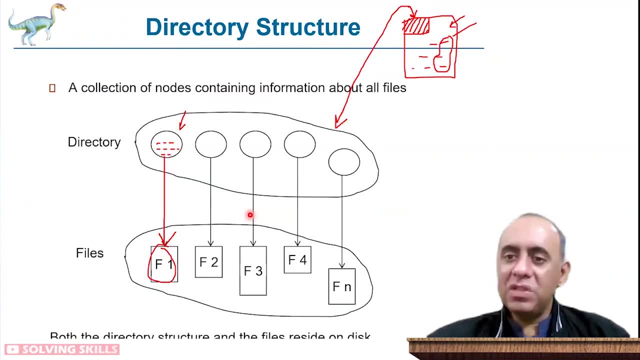 the user copied this file from this to this, but you physically didn't make a physical copy on the logical blocks of the of this file. so, for example, this was the 500 megabyte file. you didn't physically copy all these blocks over to some other location inside this, your 970 gigabytes area. you simply 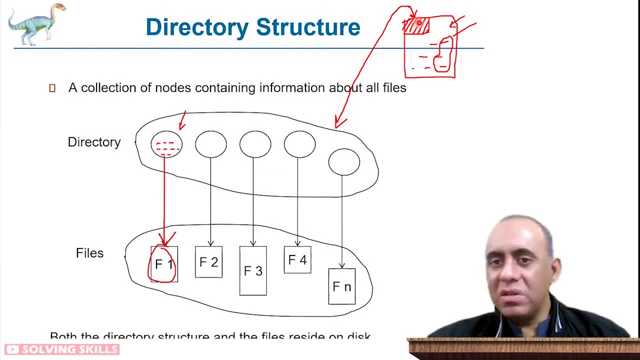 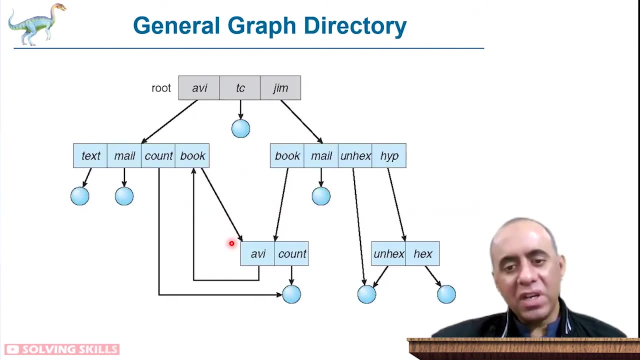 copied the address in this location to using a couple of bytes, so the file is simply copied. so there is another option that, uh, what if this collection was modified? then obviously you will have to, you know, maintain an information. this is a general graph directory, so any, any arrow is possible going from any. 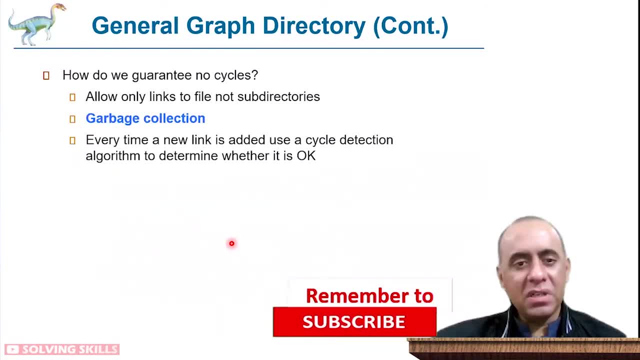 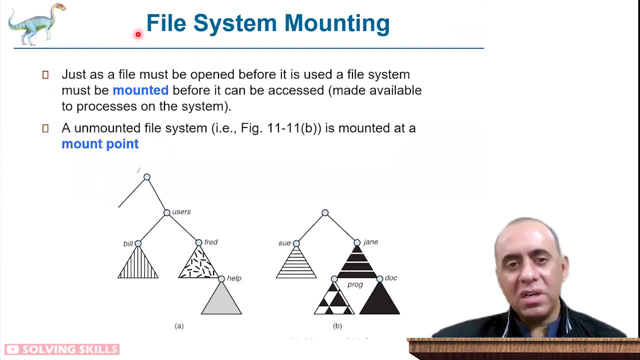 location to any other location. so these are different types. uh, yeah, so there are. so these are methods to reduce or to eliminate cycles inside the general graph directory. again, as I said that cycles may not be really useful, so we uh, delete the cycles. so this is another thing which. 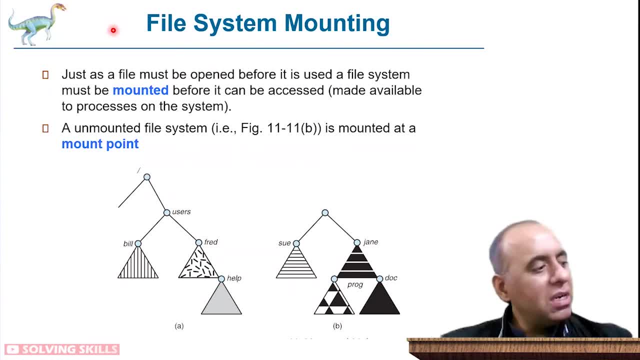 is called file system mounting. so let me show you. this is something. uh, this is a, an external hard drive, right? so just to you know, uh, jog your memories a bit. so this is a, this is a hard disk drive, this is, you know, external drive. so you connect it with this, what we call the USB, uh, 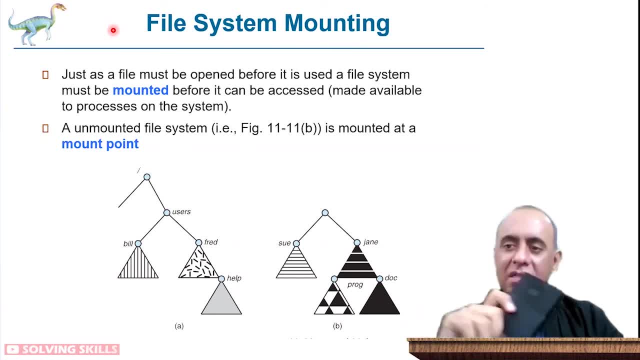 cable. so do you think? as long as this, this is in my hand. so does this contain a file system or not? on on a table, it contains a file system, but that file system can only be accessed when it becomes part of the active file system of an operating system. so right now I'm using this Windows session. 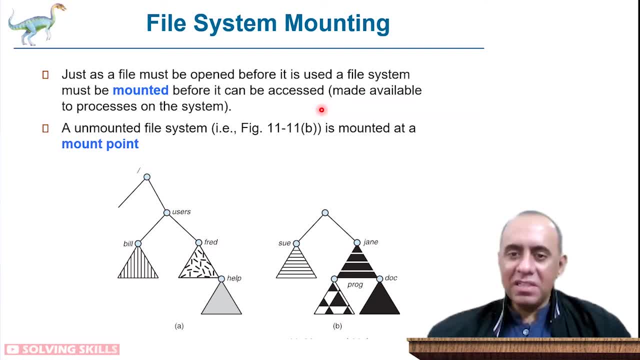 and this Windows session is an active session where the file system is also loaded inside the memory of this operating system so that it access. it can access any disk which is connected to this computer right now. so as soon as i connect this external hard drive to my computer, that file 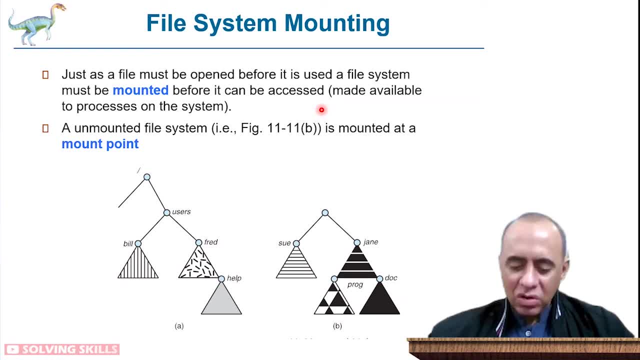 system will be. will you know, if i want to access that file system, i will have to make that file system part of my existing file system, of my operating system, which is running, uh, as i'm using the computer, right. so the process of attaching or, you know, adding a new disk to my, to my operating 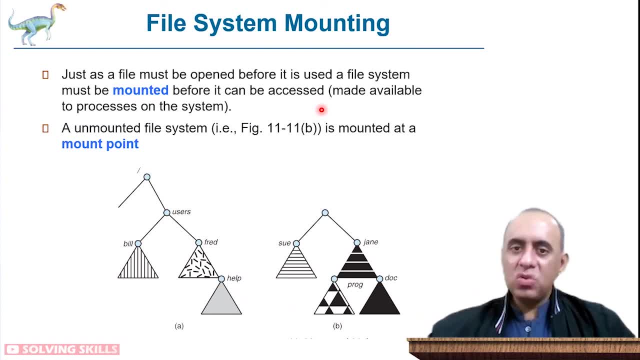 system, file system, is called mounting. so whenever i insert any- uh you know, for example, i have this thing. this is also a tiny disk in my hand, right? so this is a memory card. so as soon as i you know, so let me show you actually. so if in case of windows it is much easier because they have 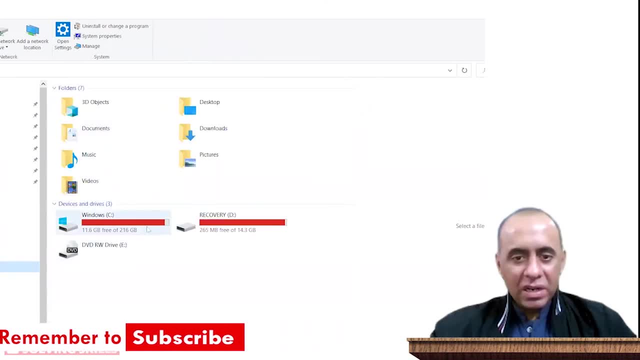 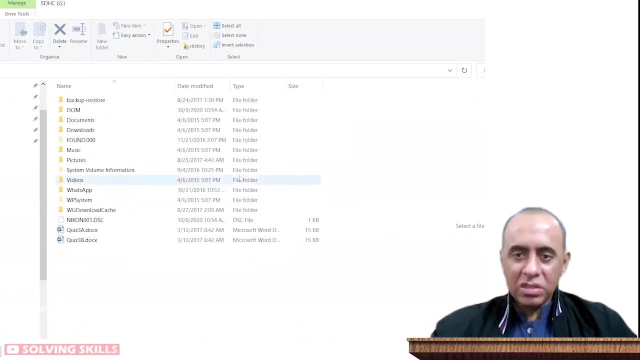 really done it in a good way. so this: these are my disks right now and they are full, by the way, and so as soon as i insert this, this memory card, inside the, inside the system, it is going to be mounted and made part of the. you know this. so here you can see this is a new partition g. so what? the operating. 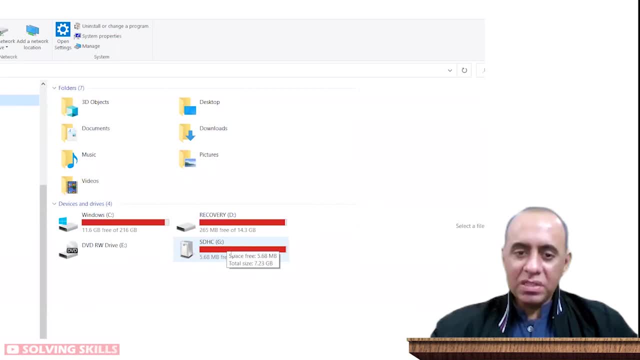 system did right now. it mounted this operating system, this file system, with the existing file system. so the linux does it in a slightly different way. it uses a sub directory to show the content of this, uh, this card. it doesn't make separate partition but again it is mounting to a different. 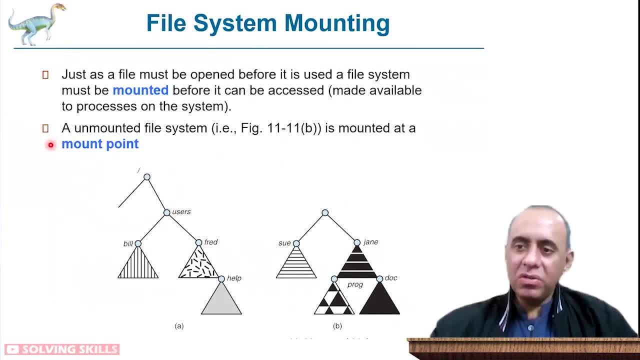 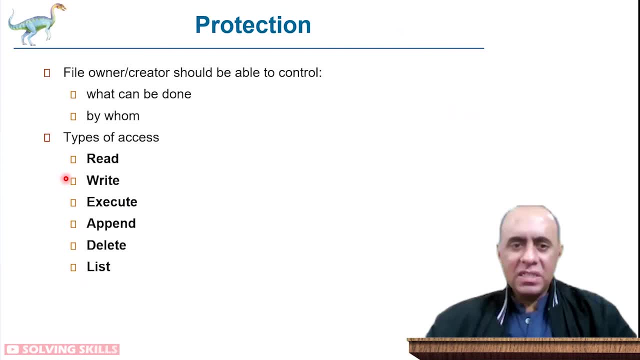 point. so in the windows mounts to the, you can say the root, there are some extended things like how to protect your files. so the file system provides, uh, you know, and obviously you could, uh, simply you could see that it's. it may not be very difficult to implement. you simply need to, uh, you know, add. 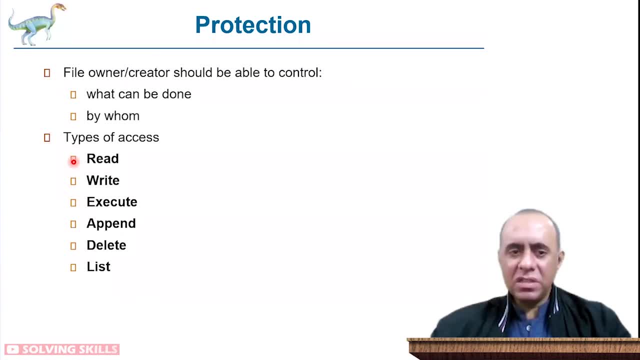 some data to your system so you can see that it's mounted to the. you can say the root. there are some uh in the file, in the directory structure. that what uh? who can access the file in what way. so these are simple checks, if else kind of checks which can be applied and similarly this is a. 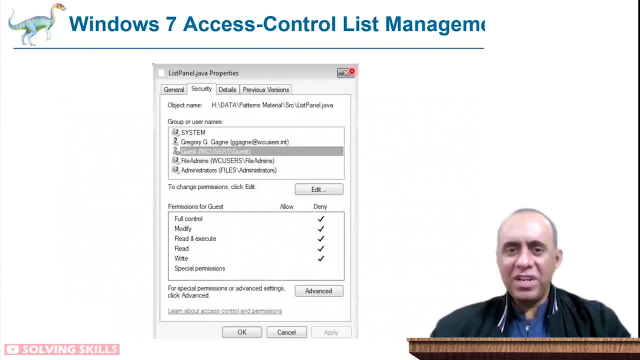 windows 7 access control list management window in which you can see that you can select a user and then you can, you know, allow or deny permissions of different types of access for that particular file for which this uh window is open. like for listpaneljava, you can select the user and you.